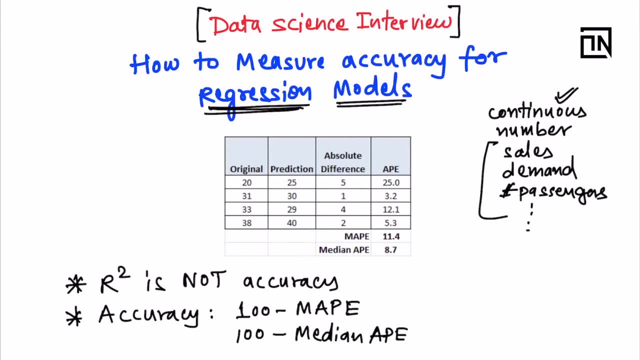 This is what I am going to discuss in this video. First of all, let me start with a common misconception: that R2 is taken as the accuracy measure, but it is not the accuracy. Accuracy is measured using 100-MAPE or 100-MedianAPE, the calculation which I am showing here in 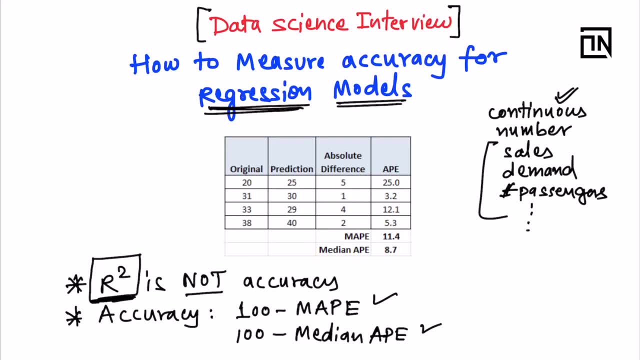 the table form. I will discuss that quickly now, But make sure that you do not mistake your answer as R2.. The moment you say I measure the accuracy of my predictive model using R2, you are clearly showing off that you have not explained it to the client. 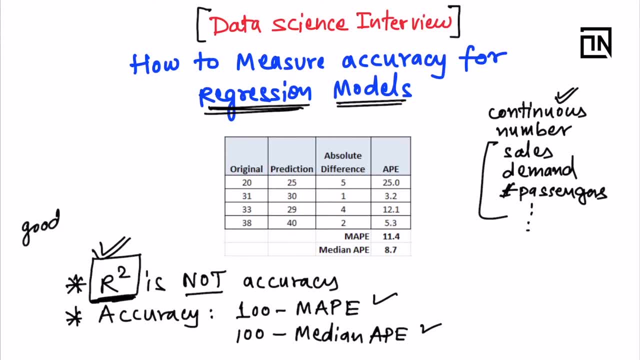 Because R2 is something which we use as goodness of fit measure And this is like fit of your training data in your model and this is not representing the actual accuracy which you test on the testing data or the validation data which you keep aside to see whether the model has really understood the patterns or not. 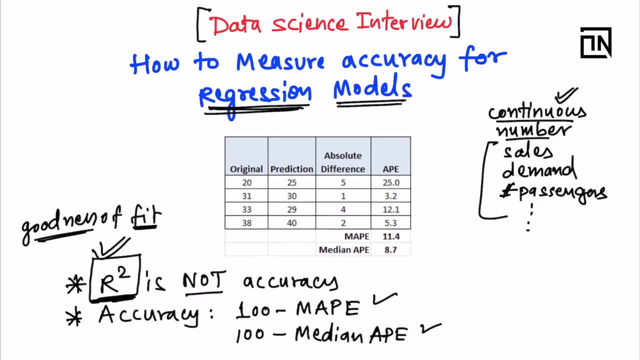 So, since you are doing a continuous number prediction, like in this scenario, you can see there is an original column and there is a prediction column. So the original column was already present and the prediction column is something which you have generated based on your machine learning. 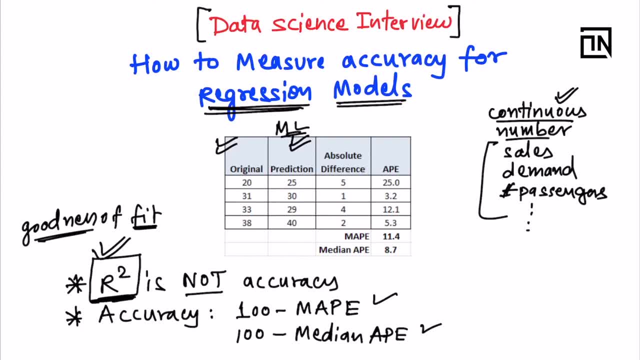 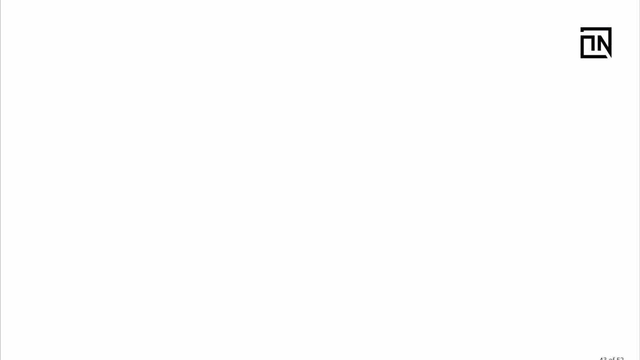 This is generated by machine learning. But where is this being generated? So first let us talk about these, from where this original and prediction is coming. So, whenever you do machine learning, you have total, full data with you, all the historical data, But you don't use the whole data in your machine learning training. 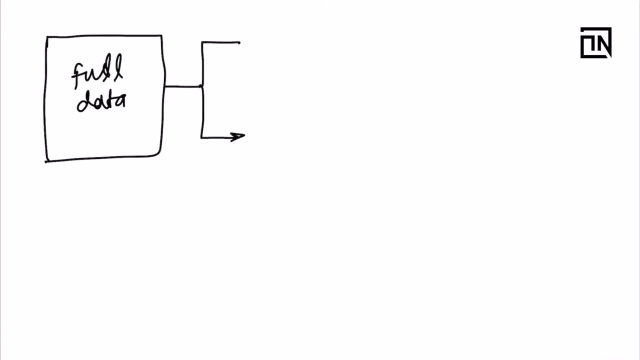 So what do you do? You split it. You split it into train, Train portion and test portion. A significant amount of data is training. So let's say a common split is 70% training and 30% testing. You can do 80% and 20% also. 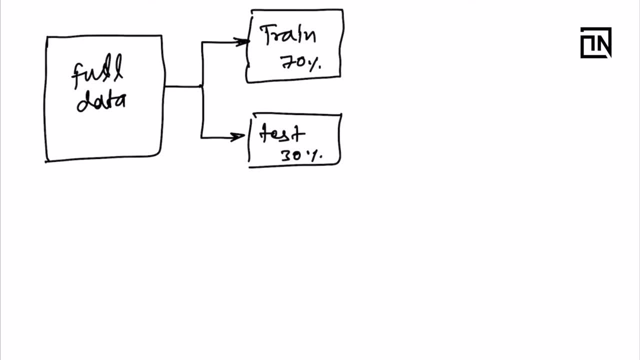 It's all about sampling theory. So you randomly sample the data, Some of the rows you keep in training, some of the rows you keep in testing. And why do we do this? We do this to check whether our model is able to understand the data. 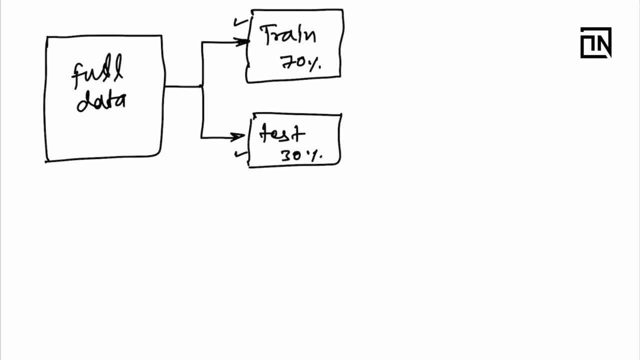 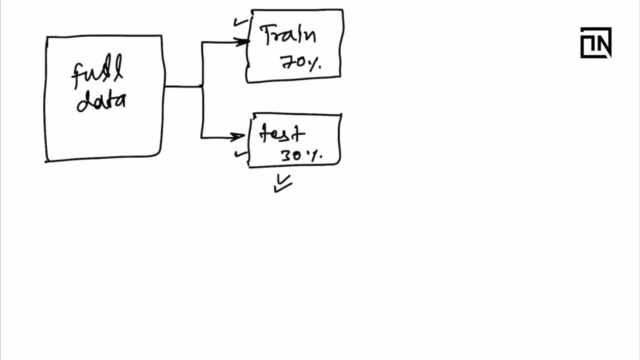 We do this to check whether our model is able to understand the data patterns in the training data or not. We test it using the testing data. So if I just mark down one more column over here and call it my target variable, which is like what you are predicting, 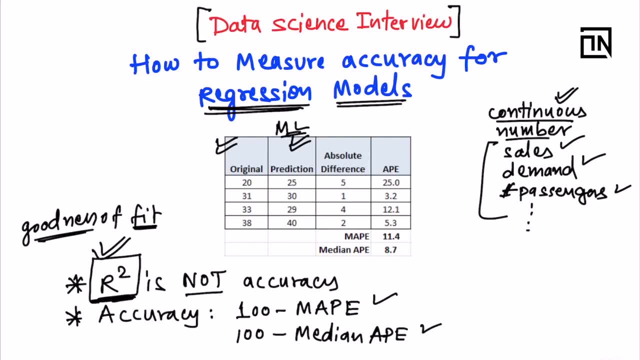 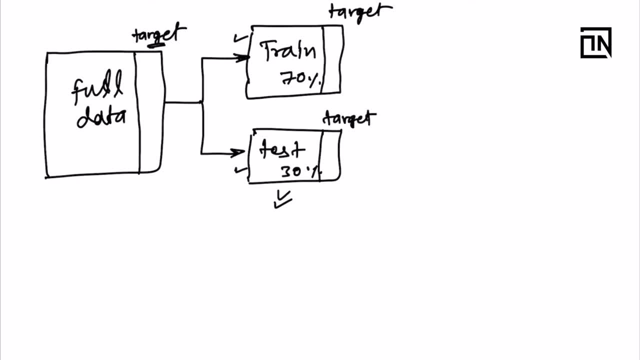 So your sales or demand or number of passengers, the target variable which you are trying to predict, it is present over here also and over here also. Okay, So the whole data itself has been splitted into training and testing. So, using the training data, I learn the patterns, I create my machine learning model. 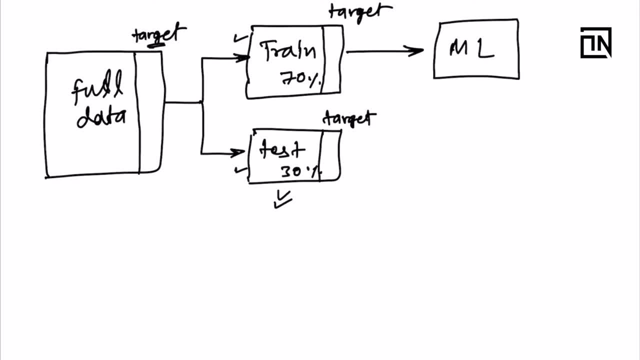 And then, once I know this, that these are the patterns, I have understood this, So I'll pass out my test data to it. So this target portion. let me rub this target portion and bring it over here. This is nothing but my original. 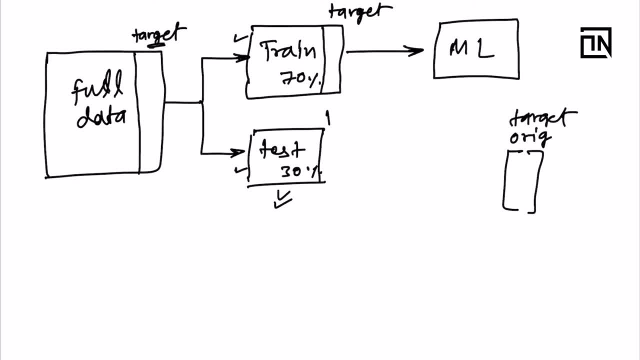 Okay, Okay, I know the answers, I know these values, So I have sent these testing target values over here and, using machine learning, So I pass this data to machine learning algorithm and this produces some result. And what is that result? This is nothing but prediction. 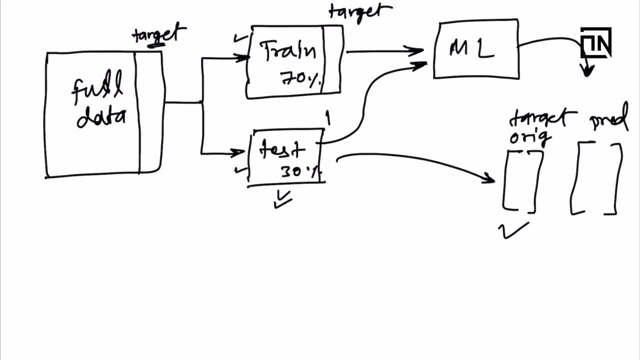 Yeah, So this original is something which I know that this must be the answer, and prediction is something which I have generated using my machine learning model. Okay, And then I'm going to compare. Okay, So this was the original. This is the prediction. 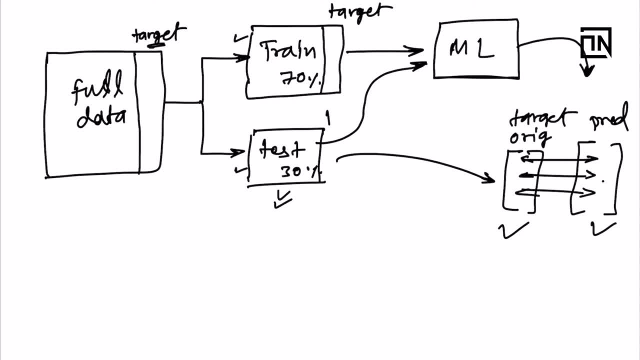 How far away these values are. Okay, Now, during the hyperparameter tuning of algorithms, while we are training, common values are utilized, such as RMSE, RMSE, MAE, etc. But these values are highly affected by the scale of the data. 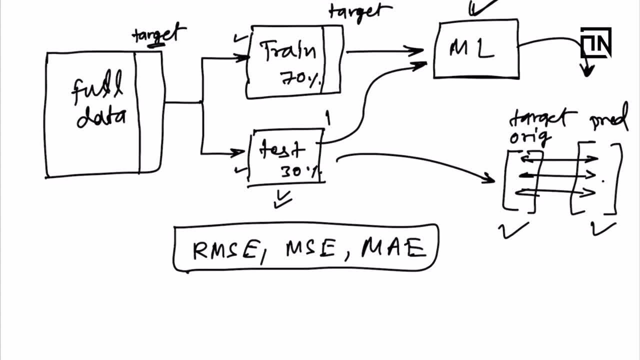 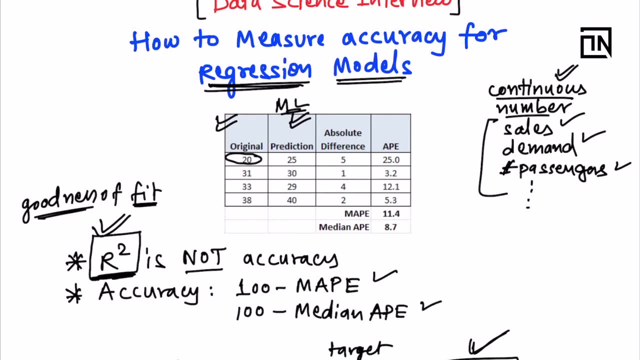 So if you try to explain the accuracy to the client, In the end what happens? What happens In the end, what your client is going to see is this table that, let's say, original value was 20 and what your model has predicted, 25.. 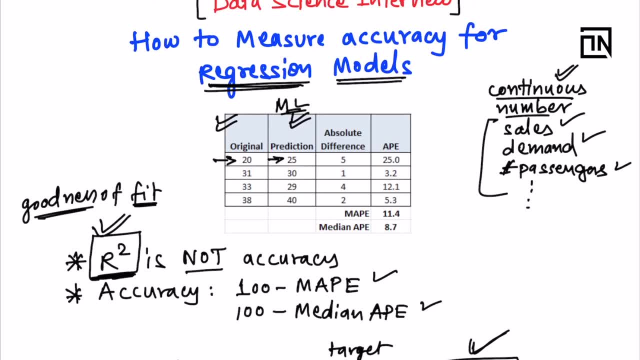 So how far away this 20 is from 25? You will say, let me compute the percentage difference. So how do we compute the percentage difference? 20 minus 25 divided by 20, this whole thing multiplied by 100, take the absolute of it. 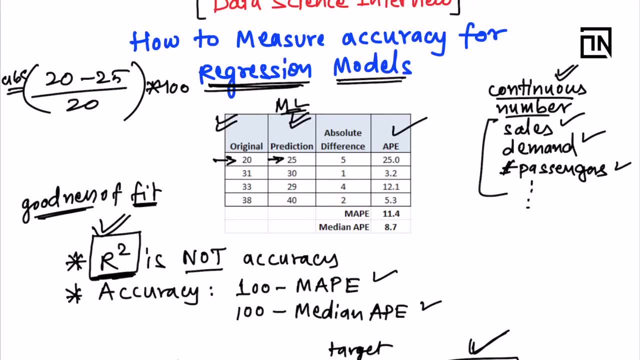 So this is nothing but the absolute percentage error which we calculate. So I say: 25 is 25% far away from 20,, 30 is 30,, sorry, 3.2% far away from 31,, 29,. the prediction: 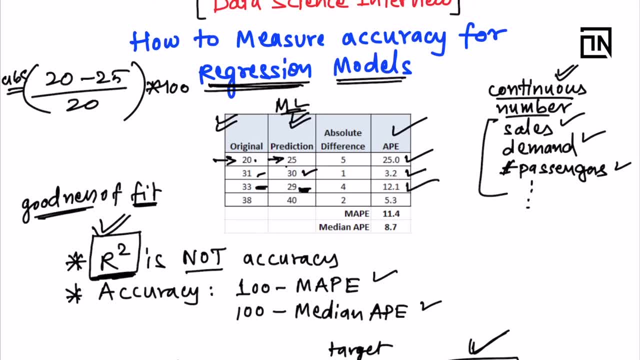 is 12.1% far away from the actual value 33.. So how far away the prediction is from the actual value or the original value? This is what I'm measuring in absolute percentage error. In another words, you can say that in every prediction, this is the amount of error I. 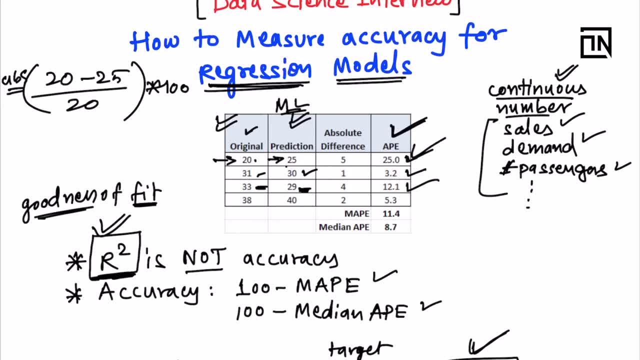 am making Like here in the first row, I'm making 25%, 3.2%, 12.1% error, 5.3% error, so on, so forth. So if I have to tell my client that how accurate my model is, what I'll do is I'll try to. 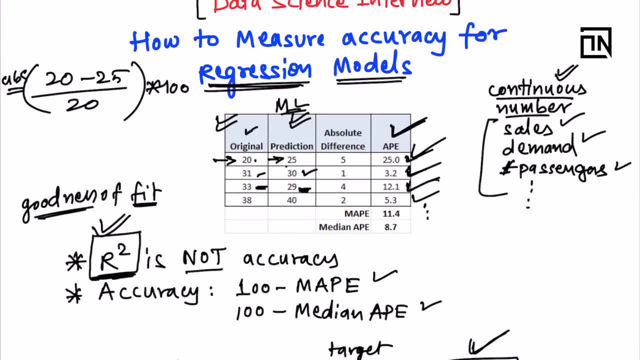 calculate on an average how much error I am making. So this is that value. the MAPE is that value which is nothing but the mean of this whole column. So 100 minus this MAPE- This becomes my accuracy And this is what I have described here. that 100 minus MAPE will give you that this is: 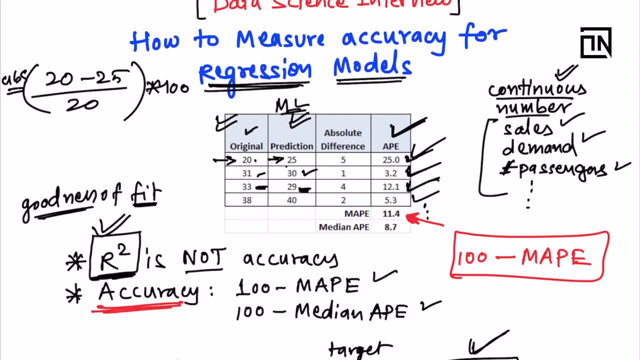 on an average how much your model is accurate, because you are subtracting the error portion from the 100 value. Sometimes this MAPE would be really huge due to the presence of some outliers, and absolute percentage error would be really huge. So what we look at, we look at the another measure of central tendency, which is median. 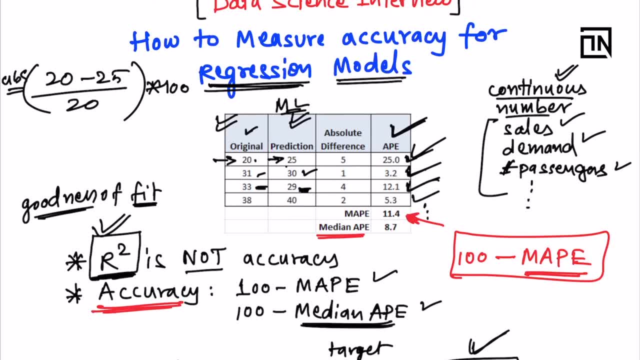 value 100 minus median MAPE. So both these measures are looked into, while describing the accuracy to the client And in an ideal world where your errors are not having any outliers, your data is good. mean absolute percentage error and median absolute percentage error. they will come. 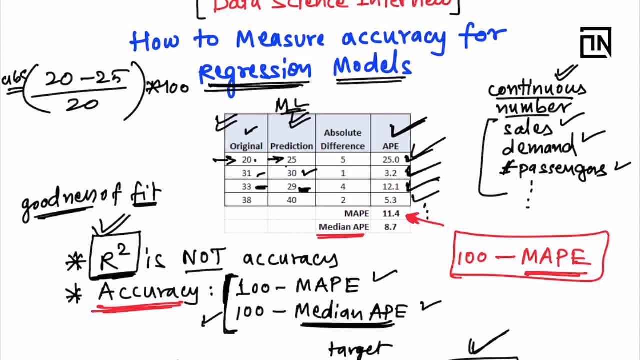 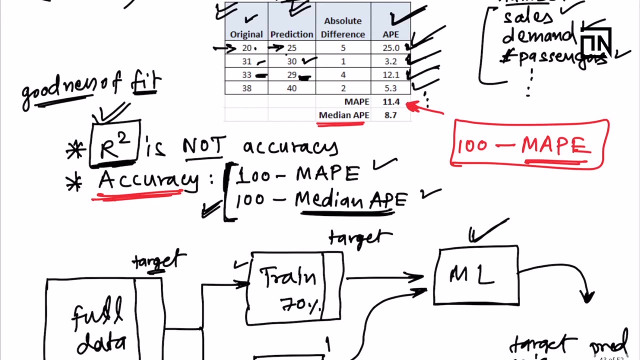 really close and the accuracy for both these terms will be similar. So this is one way, And this is majority of the places. In majority of the cases, clients would understand this terminology and they will be able to appreciate it. If you give them the RMSE value, MSE value or, let's say, the R squared value, you are 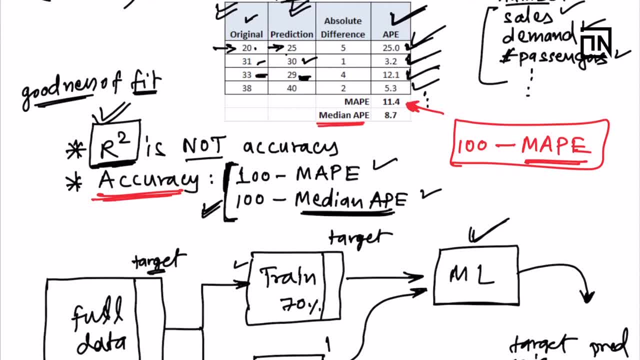 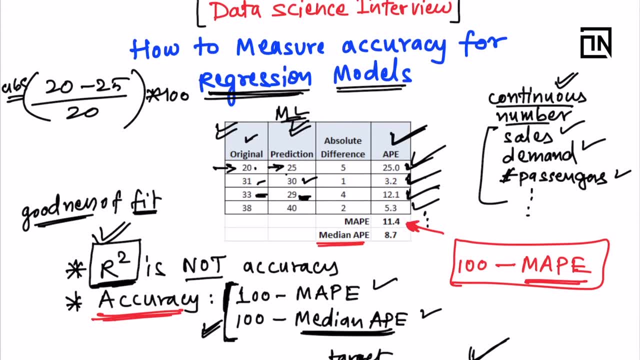 not giving them the exact way to measure how accurately the model is performing. So, in order to make it simpler for the client, we use this metric, which is MAPE. All right, Because this is a scale less metric, it works for every scenario and it is just measuring. 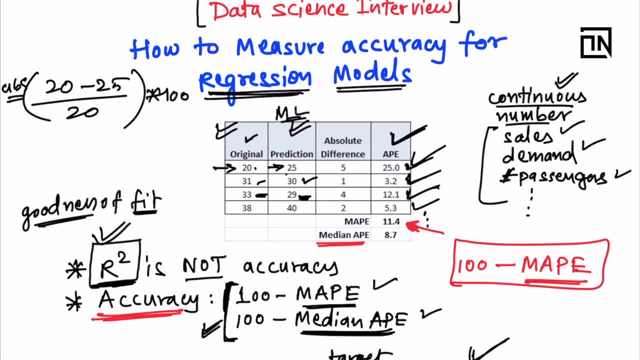 that this was the original number and how far away your prediction is from the original number. All right. Now, in some cases, I have also seen the clients utilizing their existing data using bias. So what is bias? So they try to measure the accuracy using bias. 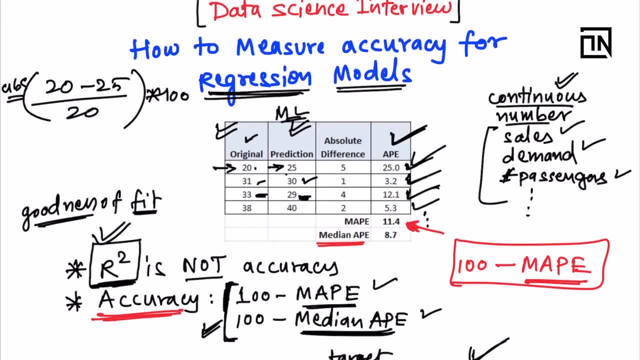 For example, here, if you take a look, take a look into the four rows of prediction which I have tabulated and if you sum this up like 20,, 31,, 33,, 38, so you can get an overall summation. 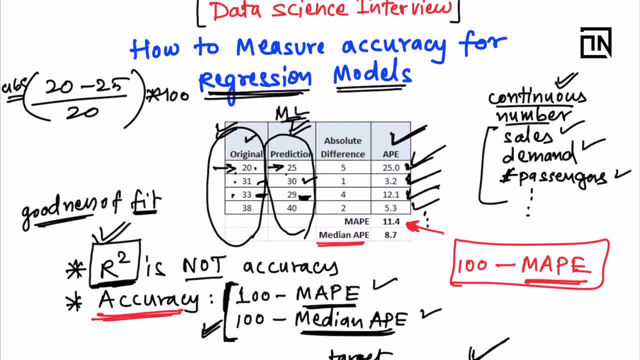 of this column. Similarly, you can get an overall summation of this prediction column. So, for example, 20, uh, 20 plus 31 plus 33 plus 38, how much, uh, how much that evaluates? So I've I've done that already. 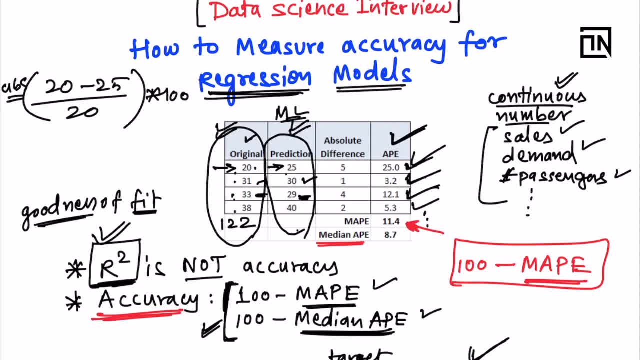 So it is. it evaluates to 122.. And if you add up the predictions like 25,, 30,, 29, and 40, how much it adds up to? So it adds up to 124.. So now this overall sum is measured. 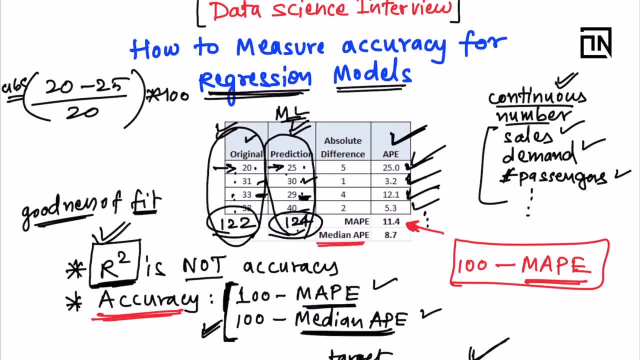 Um, As a, as a deviation or as a bias? Okay, So now I will. I will collectively try to measure that, If I sum up all the prediction versus the sum of all the original, how far away these two numbers are. this is nothing but my bias. 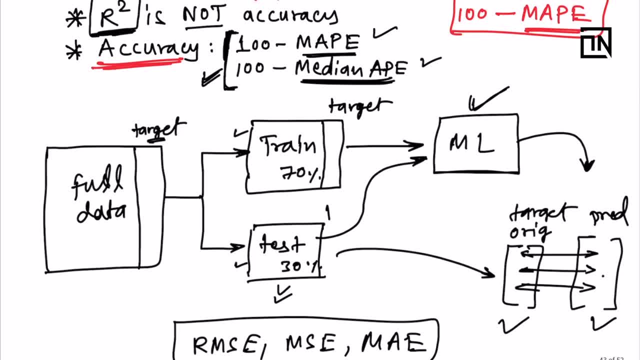 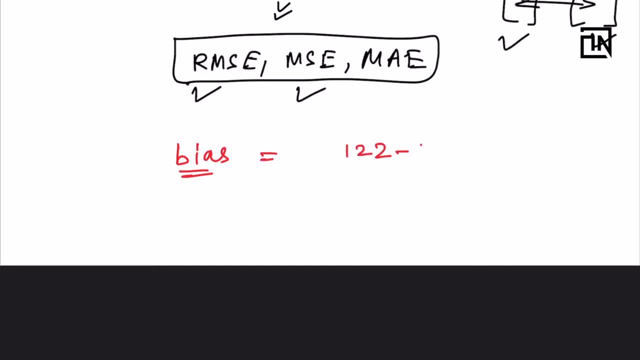 Okay, So how then I will calculate the bias? Bias will be once again calculated as uh 122 minus 124.. This is the sum of original, Okay, And this is the sum of prediction, And then divided by original reference, sum of original, which is 122. 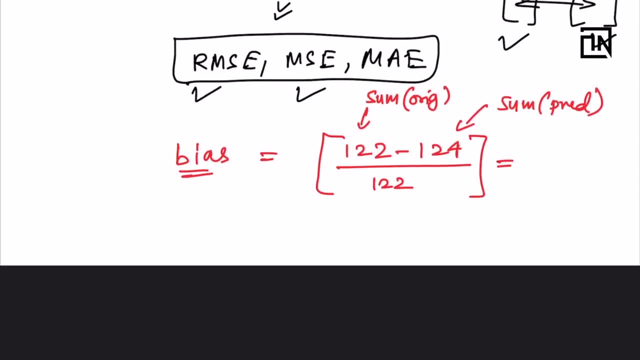 Okay, So this will produce me. uh, let's say this is going to give me 1.63 minus 1.63. So this is nothing but the difference and I take the absolute value So 1.63.. So 100 minus 1.63, this becomes my accuracy. 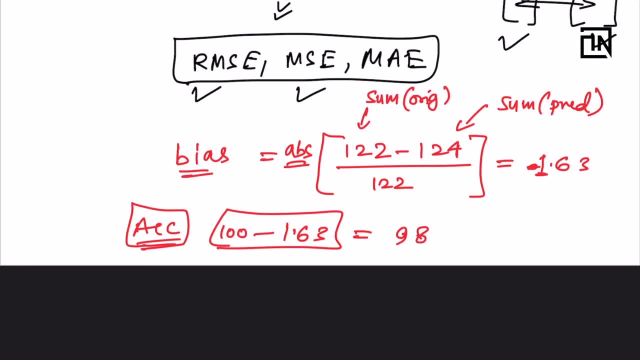 So I'll say my model is uh 98.36 accurate. So all in all, like if you take the summation of all the original and summation of all the prediction, how far away they are from each other. So they are 1.63% far away from each other. 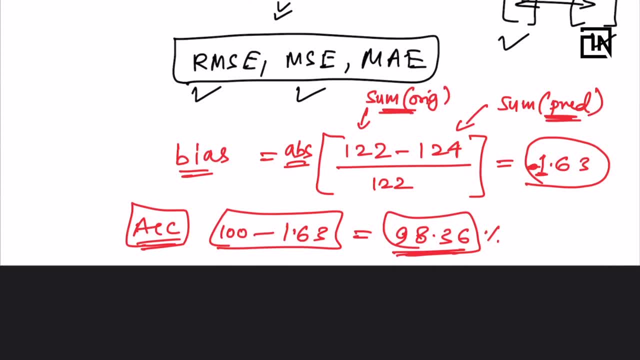 So if they are far away, 1.63%. So how accurate? my model is 98.36%. So this is also known as bias, and it is also utilized in some of the scenarios, although it has its its own demerit, because in some cases it will simply add up the uh problems. 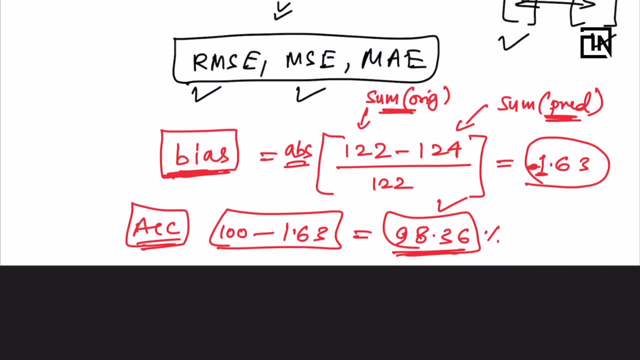 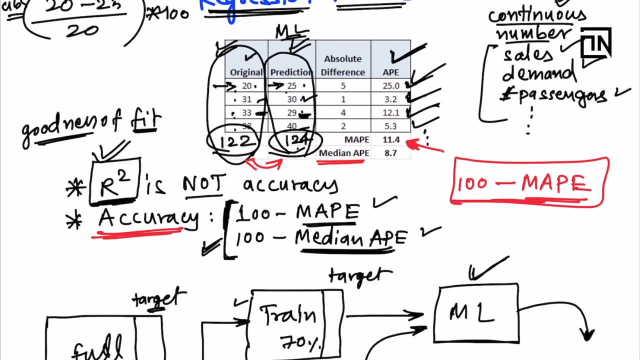 and overall impression would be of a highly accurate model. If you see in this scenario itself, uh, the the accuracy based on a hundred minus MAPE would be somewhere around uh 88% and based on bias it is coming as 98%. 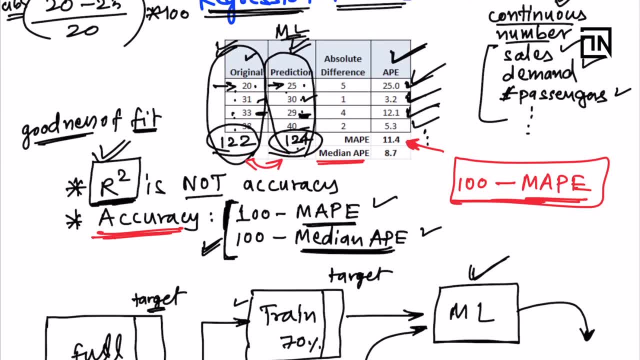 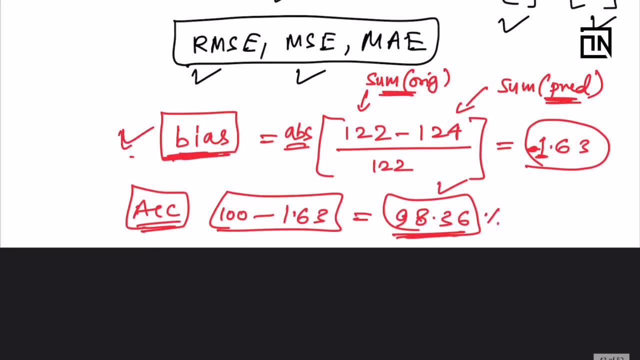 So 10%, 10% jump. uh, you are witnessing when you are employing bias. So bias is something which prints a very rosy picture. So that is why bias, if you are using, you must always use it in conjunction to the MAPE. 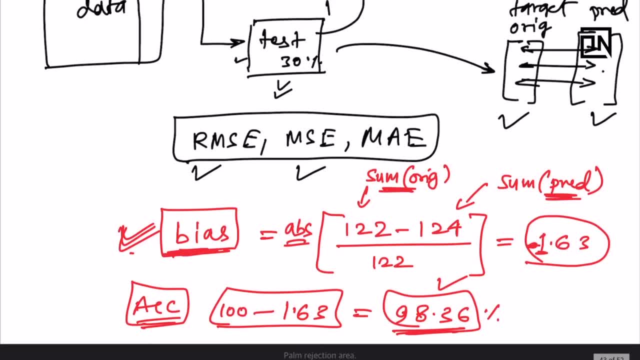 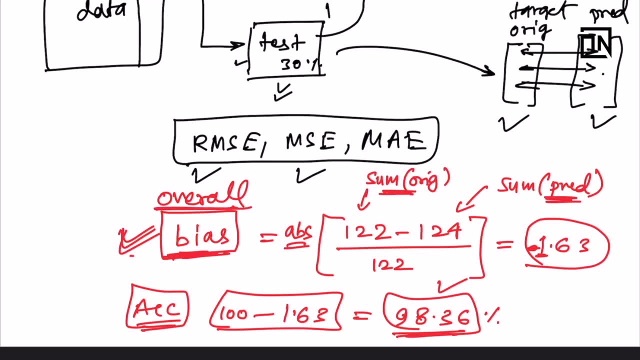 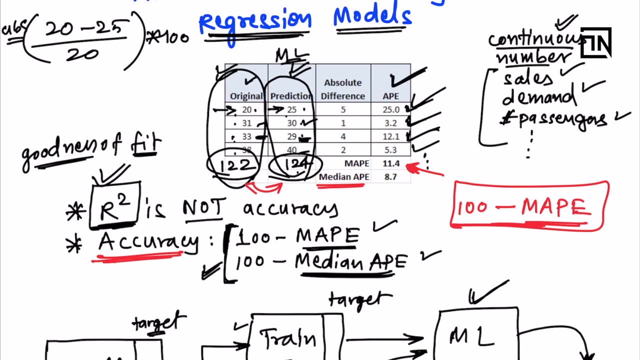 because this will give me event level accuracy or the row level accuracy, And this will give me overall accuracy. Okay, Which is which is sometimes misleading, because, uh, wherever you have made uh errors in predictions, It uh added up to where you have not made it or made the errors in the negative direction.